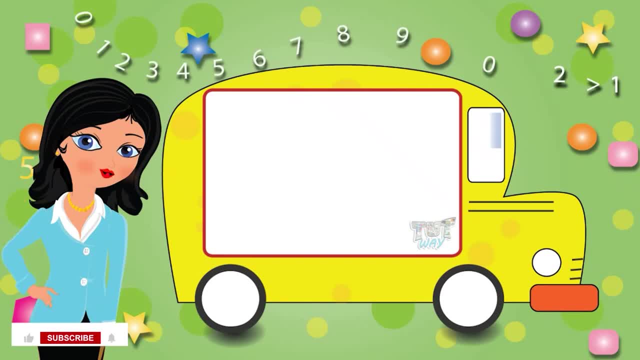 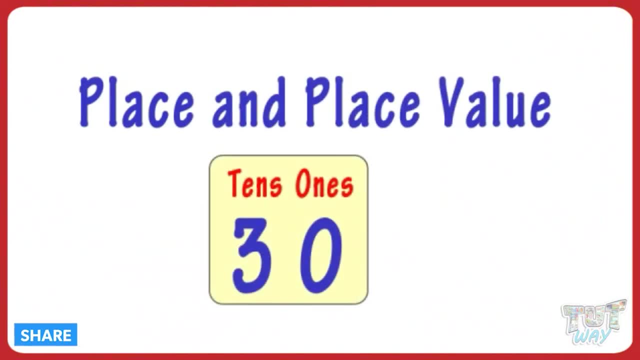 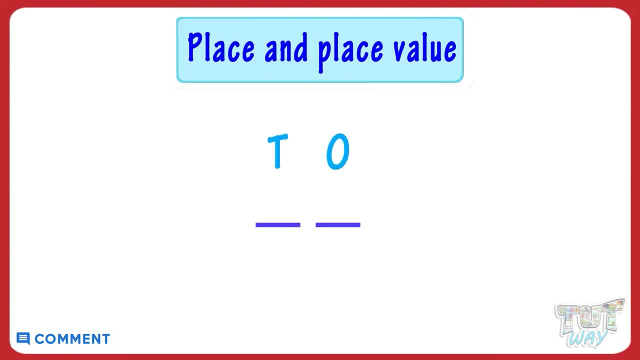 Hi kids, Today we will learn what is place and place value of a digit in a number. So let's get started. Place is the position of the digit in a number. Example: here we have a number Number. Place of 3 in this number is 10's place. 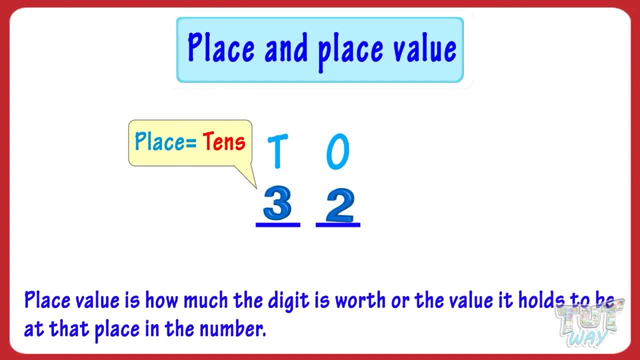 Place value. It is how much the digit is worth or the value it holds to be at that place in the number. Example: place value of 3 in this number is 3- 10's or 3- 10's Or 30.. 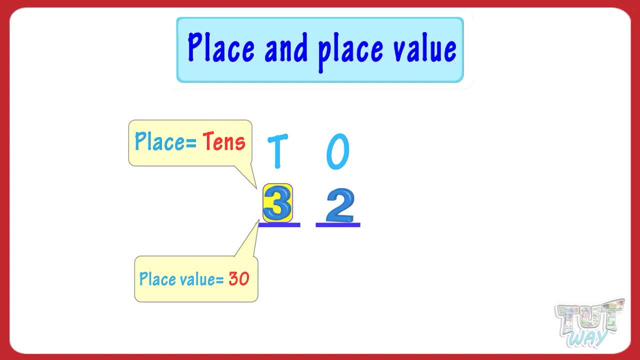 Let's learn the concept with more examples. We have a number 457.. Let's start with 7.. Its place is 1's place And place value is 7- 1's, that is 7.. Place of 5 is 10's. 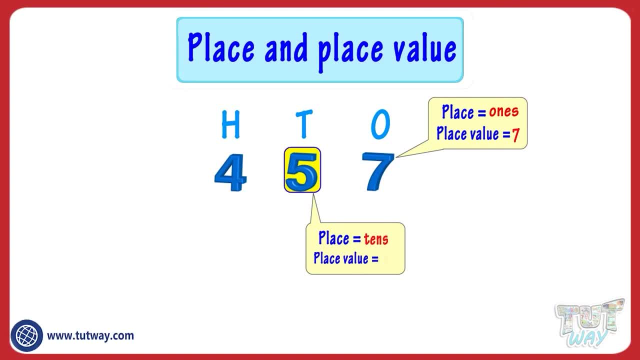 Place value is 5, 10's, that is 50.. Place of 4 is 100's. Place value of 4 is 400.. So, kids, let's take another example. Here we have another number. Now let's see the place and place of each digit in this number. 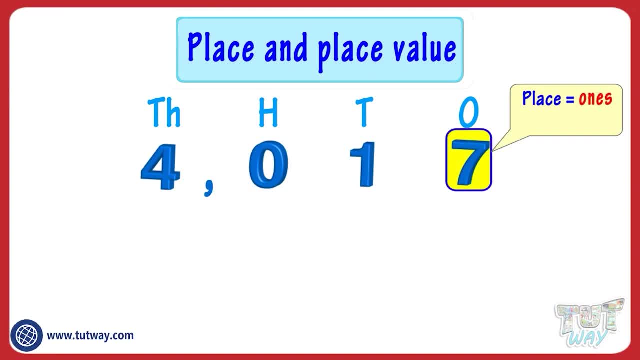 Place is 7- 1's And place value is 7.. Place of 1 is 10's And place value is 1- 10,, that is 10.. Place of 0 is 100's And place value is 0, 100 or 0..